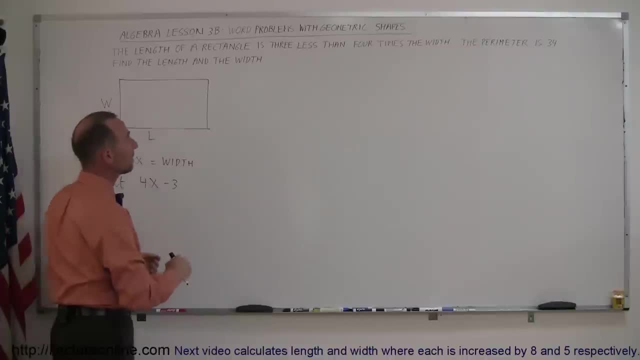 is 4 times the width minus 3, which means 3 less than 4 times the width, and that will represent the length. Alright, so now that we have both the width and the length expressed in terms of x, we can now go ahead and use the information that tells us that the perimeter 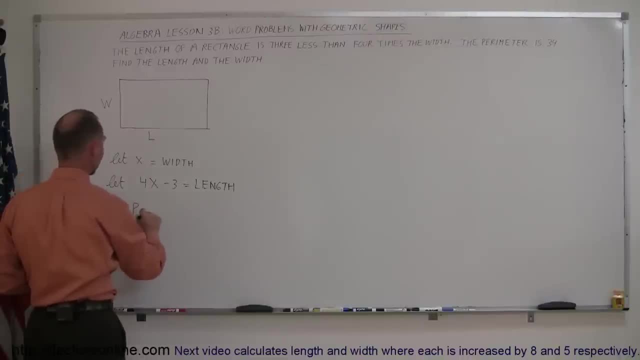 is 34.. So we can say that the perimeter, which is defined as twice the width plus twice the length, Now we plug in what the width and the length are equal to in terms of x. So perimeter is equal to 2 times the width, which is x, plus 2 times the length, which 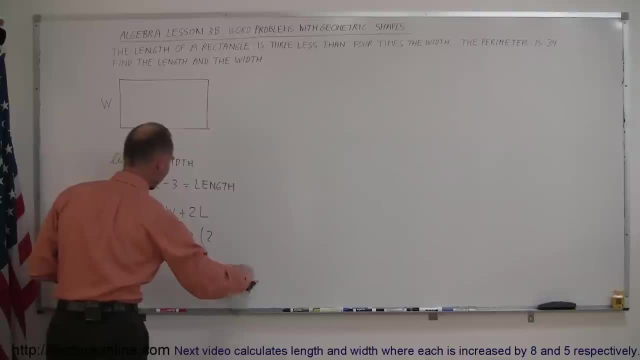 is 2x, not 2x, but 4x minus 3.. 4x minus 3.. And of course the perimeter was defined as 34, so now I can write that 34 is equal to 2x plus 2 times 4x minus 3.. And now we just 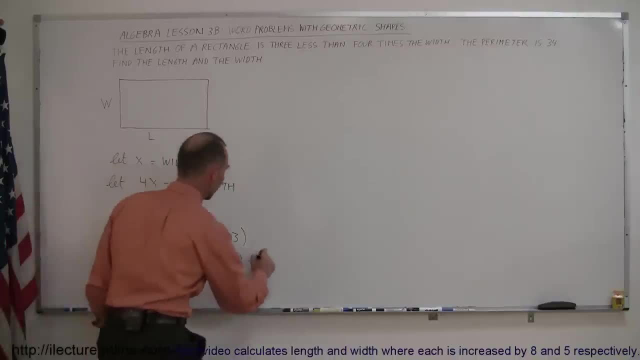 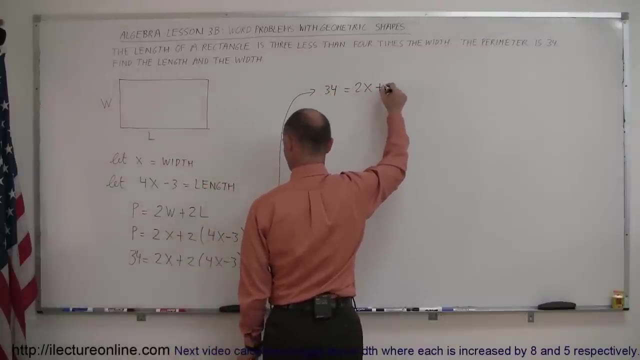 have to solve that for x. Alright, Giving myself some more room rewriting it over here, I can say that this is: 34 is equal to 2x plus 2 times 4x minus 3.. Alright, so what do we? 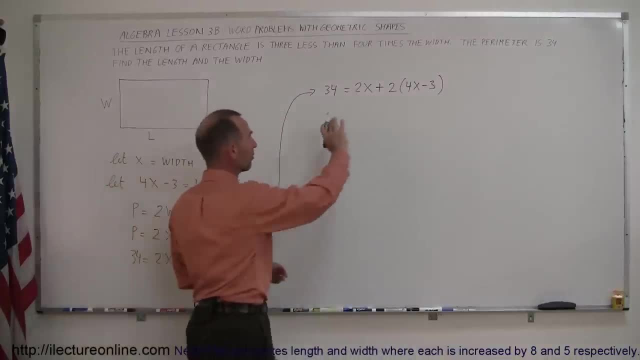 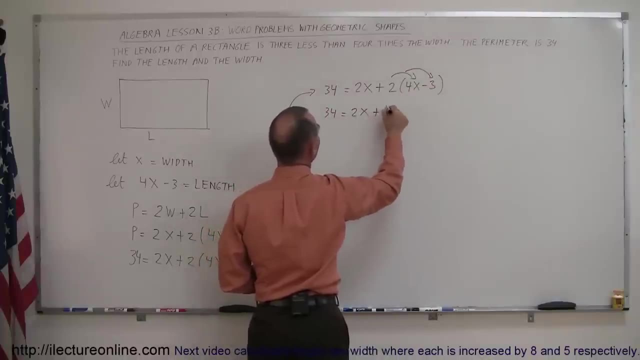 do first. Well, we want to get rid of the parentheses first, so let's multiply the 2 with both the 4x and the negative 3.. So we have 34 equals 2x plus 8x minus 6.. Now the 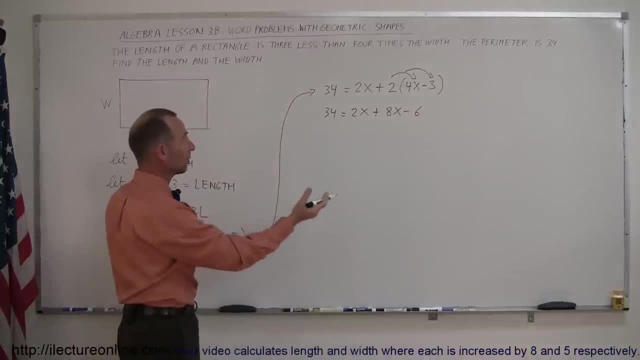 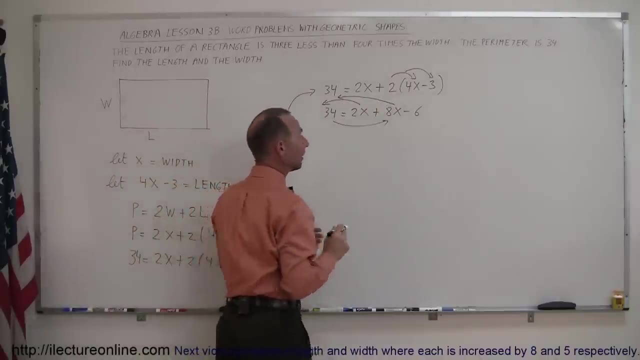 next step is to move all the terms with the x in it to the left side, everything else to the right side. So we're going to move the 2x And the 8x to the left and the 34 to the right Again when you cross the equal sign. 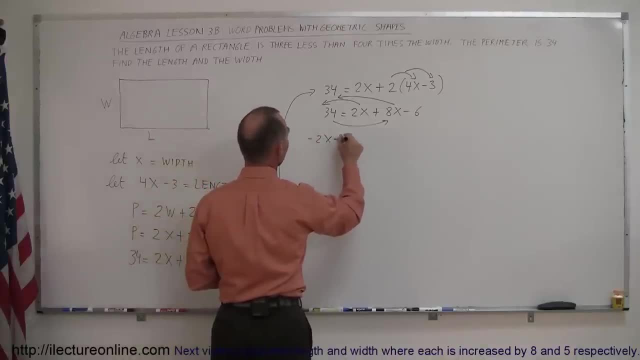 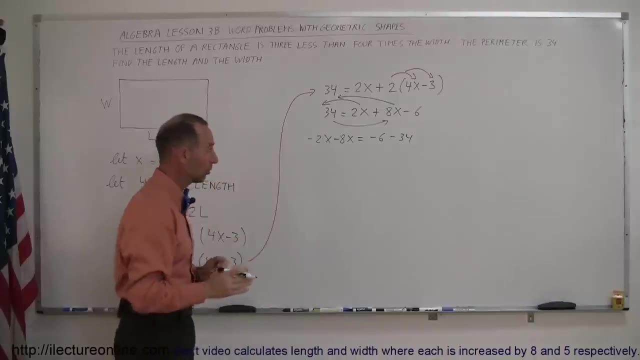 you change the sign so this becomes minus 2x. minus 8x equals minus 6, which is already, on the right side, minus 34.. Then combining like terms minus 2x, minus 10x, minus 8x is: 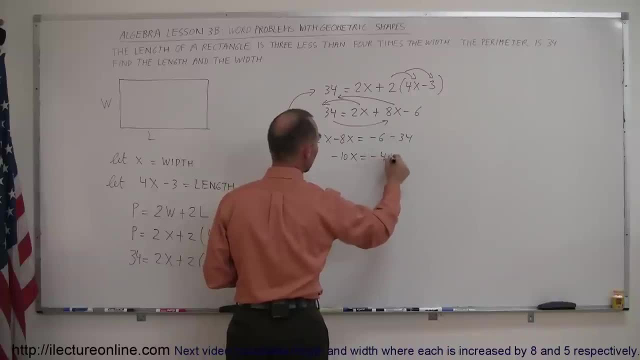 minus 10x equals that would be minus 40, and then dividing both sides by the numerical coefficient in front of the x, which is minus 10,, we get x is equal to a positive 4.. So, alright, going back to see what that means, we defined the width as x, so we know that. 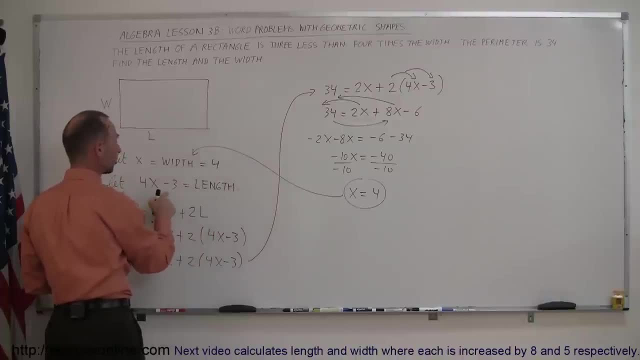 the width now is 4, and then the length is 4 times that minus 3.. Well, 4 times 4,, that's 16 minus 3,, which is therefore 13.. And there are the 2 answers: The width is 4, and the 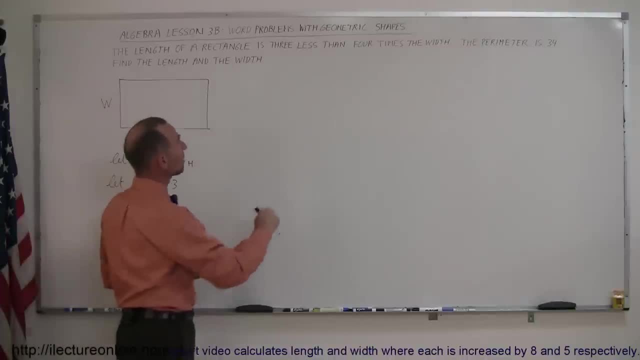 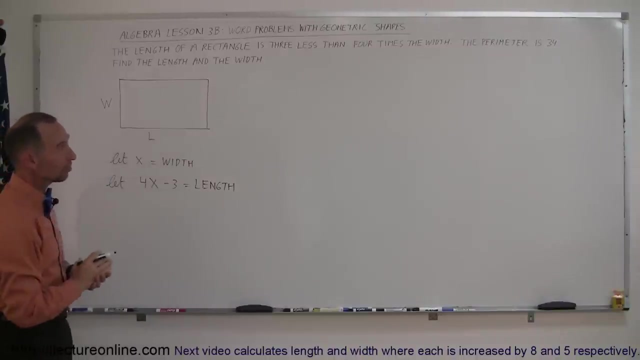 4x, the width minus 3, which means 3 less than 4 times the width, and that will represent the length. All right, so now that we have both the width and the length expressed in terms of x, we can now go ahead and use the information that tells us that the perimeter is 34.. 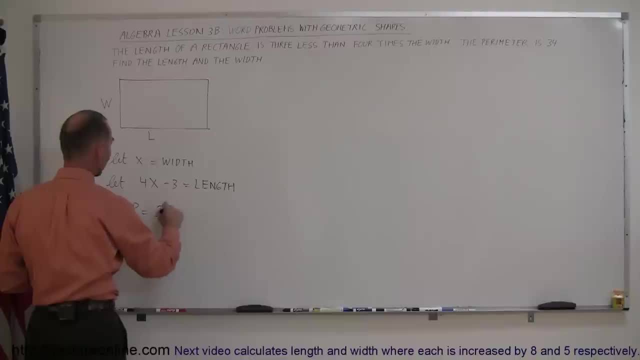 So we can say that the perimeter, which is defined as twice the width plus twice the length, now we plug in what the width and the length are equal to in terms of x. so perimeter is equal to 2 times the width, which is x. 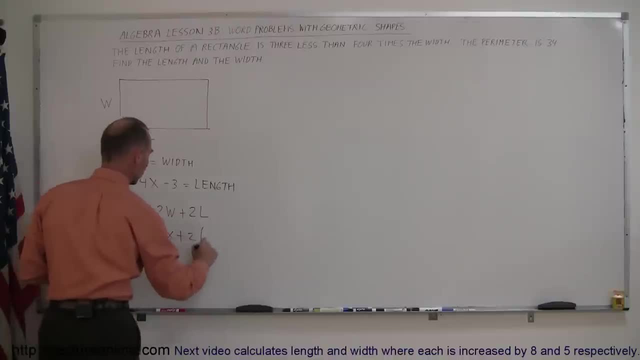 plus 2 times the length, which is 2x. oh, not 2x, but 4x minus 3.. 4x minus 3.. And of course the perimeter was defined as 34, so now I can write that 34 is equal to 2x plus 2 times 4x minus 3.. 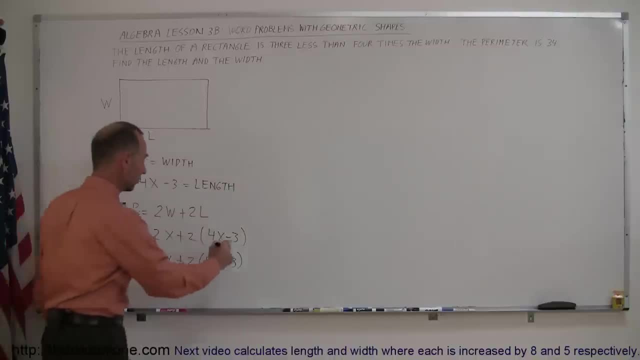 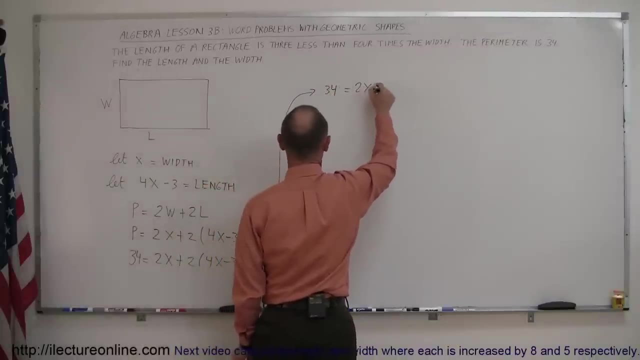 And now we just have to solve that for x. All right, giving myself some more room rewriting it over here, I can say that this is: 34 is equal to 2x plus 2 times 4x minus 3.. All right, so what do we do first? 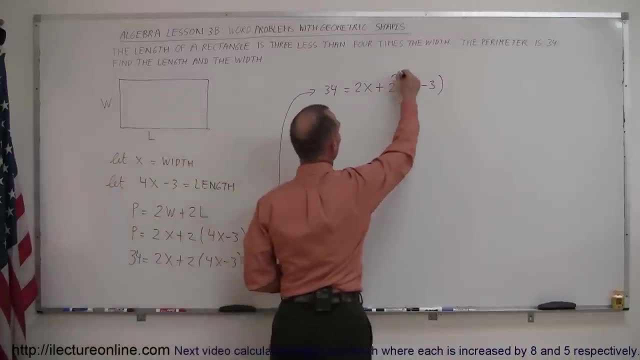 Well, we want to get rid of the parentheses first, so let's multiply the 2 with both the 4x and the negative 3, so we have 34 equals 2x plus 8x minus 6.. Now the next step is to move all the terms with the x in it to the left side. 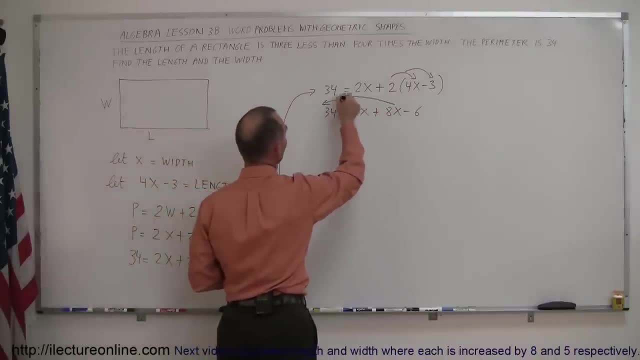 and everything else to the right side to 2x and the 8x to the left and the 34 to the right. Again, when you cross the equal sign, you change the sign so this becomes minus 2x. minus 8x equals minus 6,. 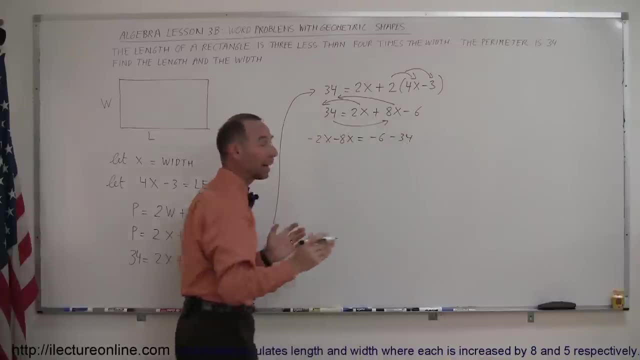 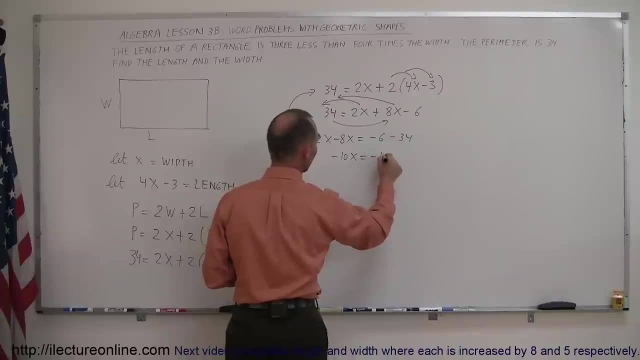 which is already on the right side, minus 34.. Then combining like terms to minus 2x, minus 10x, minus 8x is minus 10x, equals that would be minus 40, and then dividing both sides by the numerical coefficient in front of the x, 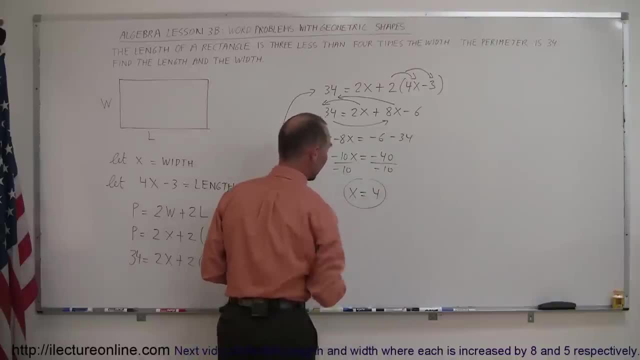 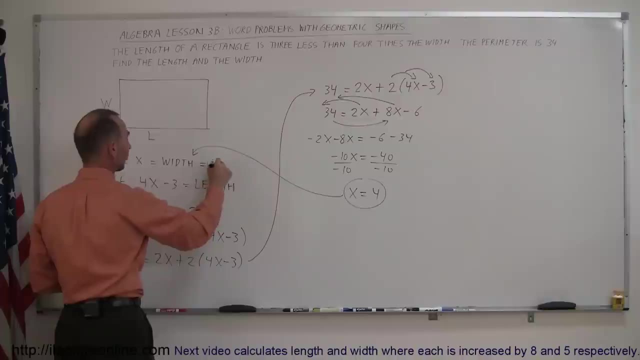 which is minus 10, we get x is equal to a positive 4x. All right, going back to see what that means, we defined the width as x, so know that the width now is 4, and then the length is 4 times that minus 3,.